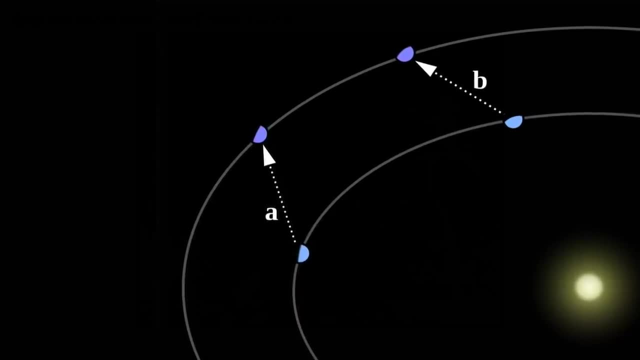 This means that Uranus is the second planet in the solar system and that Uranus is the second planet in the solar system. This means that Uranus is the third planet in the solar system. They then made some predictions and concluded the reason was because there was another planet. 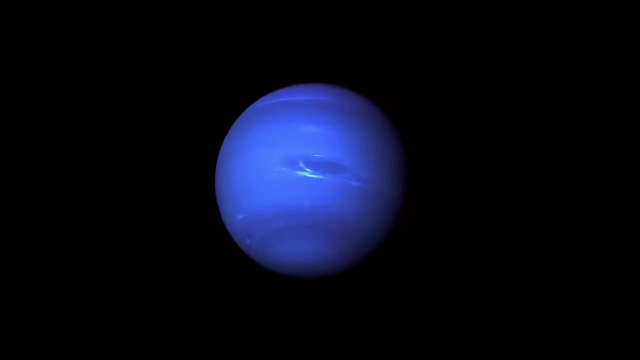 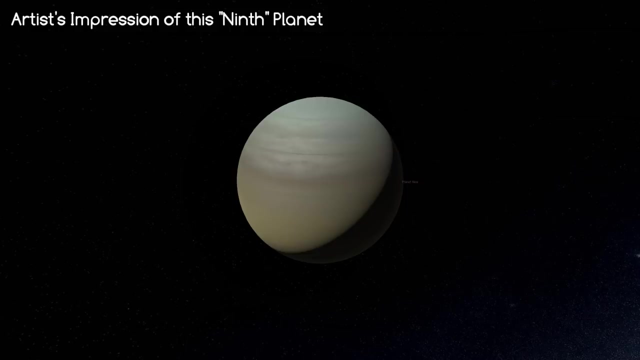 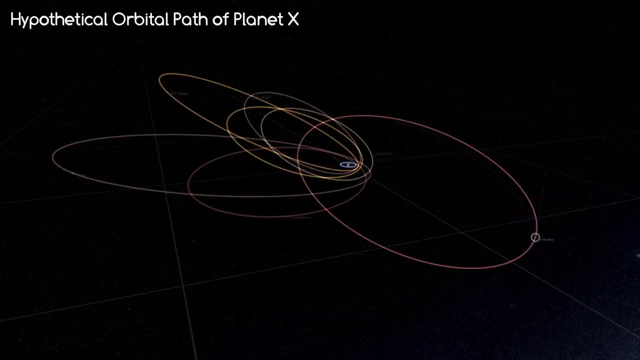 that had a gravitational influence on it. They predicted where this planet should be and, as a result, Neptune was discovered. Interestingly, the same theory surrounds this planet X, which you might have heard about this year. Some far out objects in our solar system are not where they should be, and theory suggests this is because of another planet. 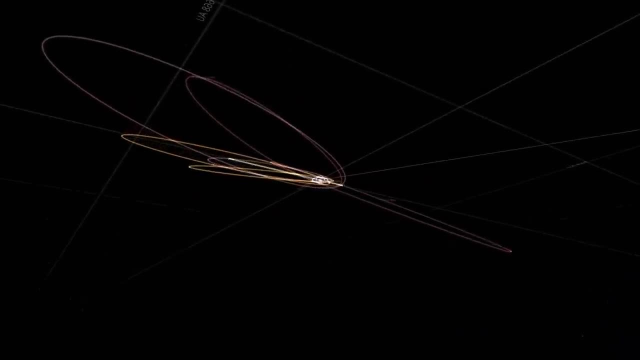 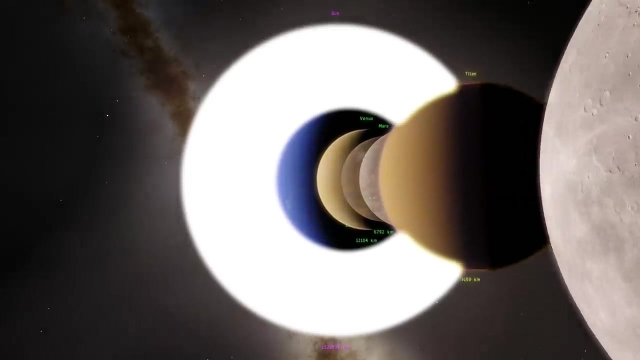 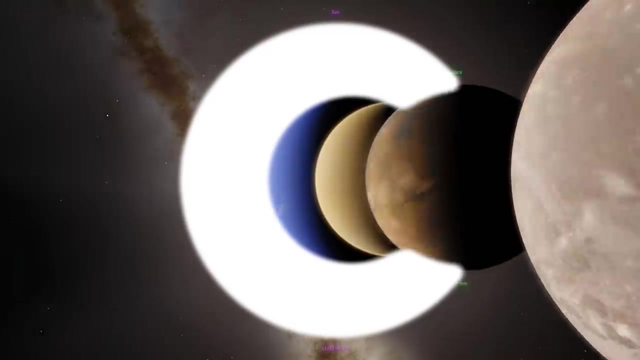 that has a gravitational influence on them. The hunt is now on to actually find this planet. Now, what's really interesting about Uranus is its rotation. Most planets rotate like a spinning top on the table of the solar system plane- Not Uranus. No, Uranus has fallen. 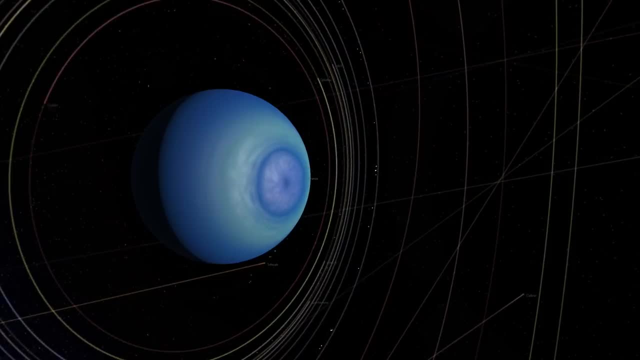 over and is rolling instead for most of its year. You see, its axial tilt is 97 degrees. This means its seasons are crazy in comparison to the rest of the planets: During its solstice or the time of the year when the sun is highest. 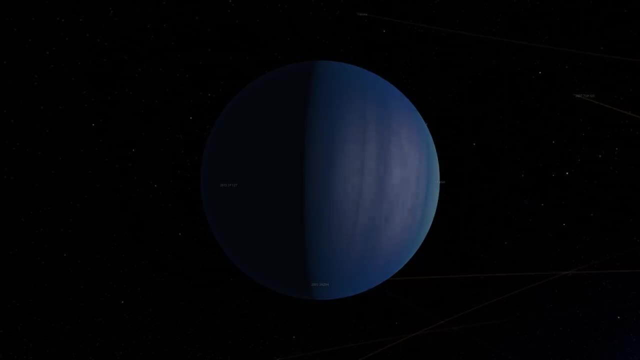 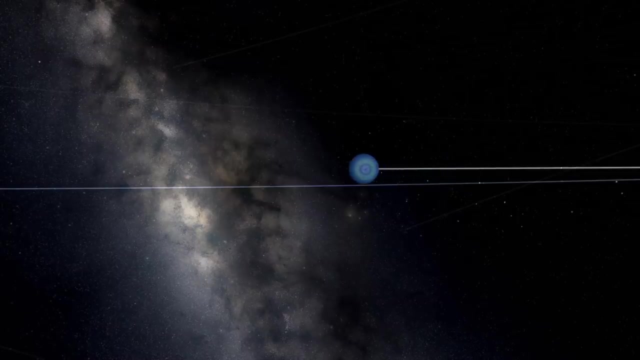 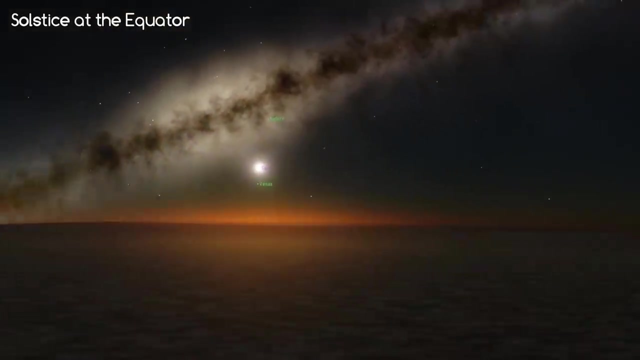 or lowest in the sky. one side of the planet always faces the sun, while the other is in complete darkness. It kind of looks like the planet is rolling forward along its orbit. Only a very narrow strip near the centre of the equator experiences day and night during. 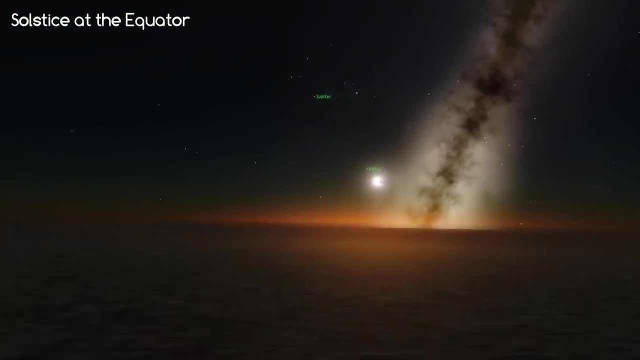 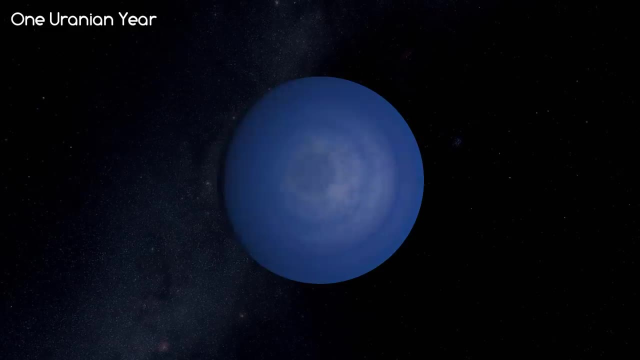 this time, but the sun only rises just above the horizon. This means that Uranus is the third planet in the solar system. This means that the sun is always on the surface. The Poles get 42 years of continuous darkness, followed by 42 years of daylight During its 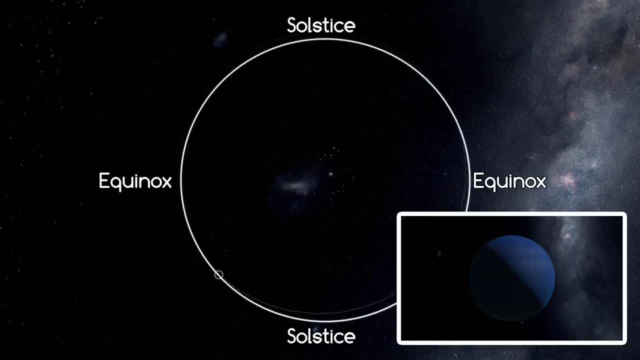 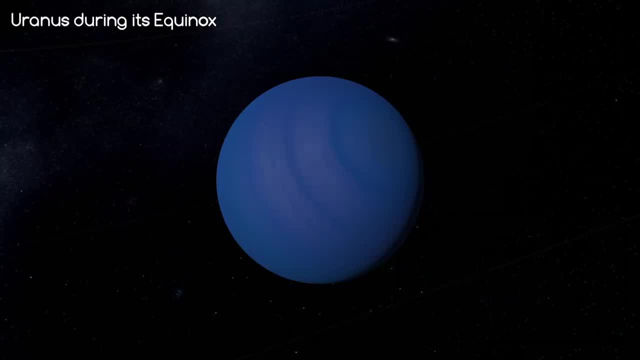 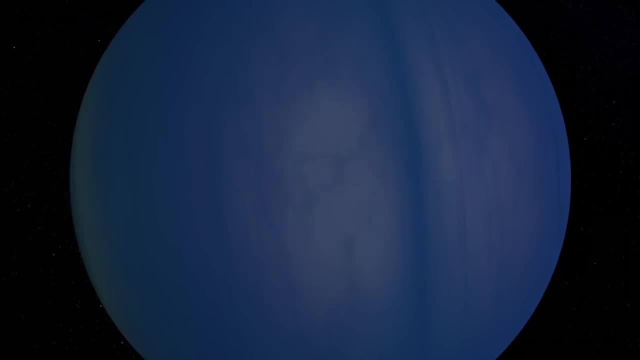 equinox, which is the opposite of the solstice. the planet has a more of a normal day-night cycle. Uranus rotates once every 17 hours and 14 minutes, but because its surface is not solid, some power lines are not solid enough to keep it on the surface. This is: 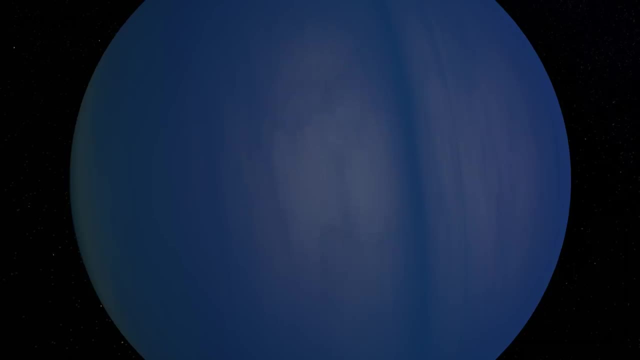 why the sun is always on the surface, and so is the light. It is called the solstice. Some parts of the atmosphere rotate faster than others and, due to high winds, some parts can make a full rotation of the planet in only 14 hours. 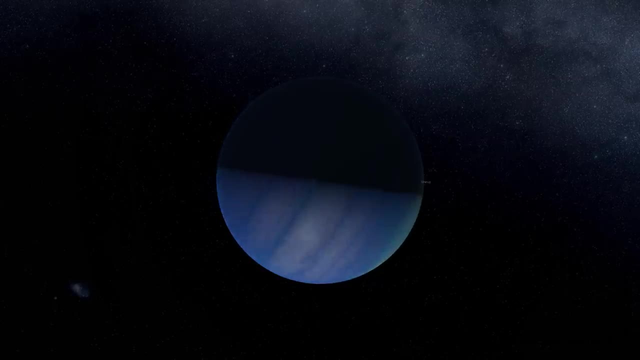 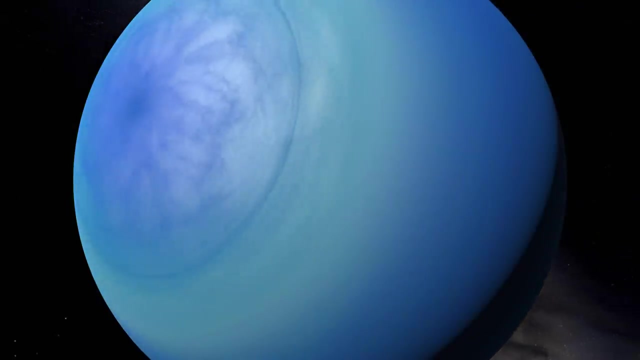 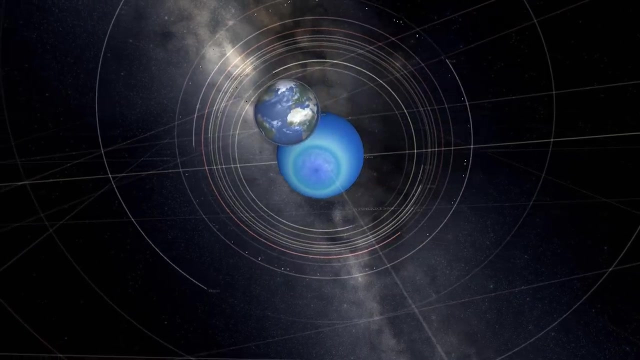 This strange rotation means it's the only planet that gets more energy from the Sun at its poles on average than its equator. For some reason, though, the equator is hotter than at the poles, and no one really knows why. Speculation also exists as to why Uranus rotates the way it does in the first place. 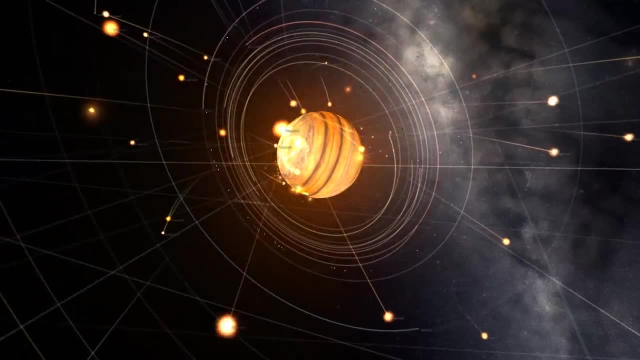 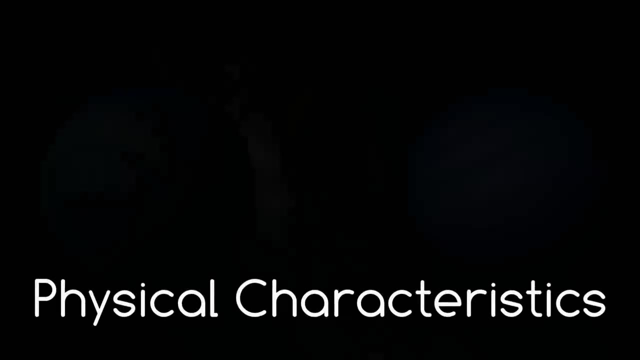 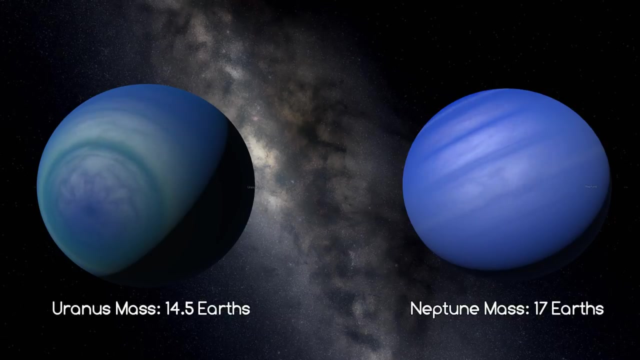 although it is generally accepted that a large Earth-sized planet crashed into Uranus, knocking its rotation on its side. So how big actually is Uranus? Well, it is the least massive of the gas giants, at 14.5 Earths compared to Neptune's 17. 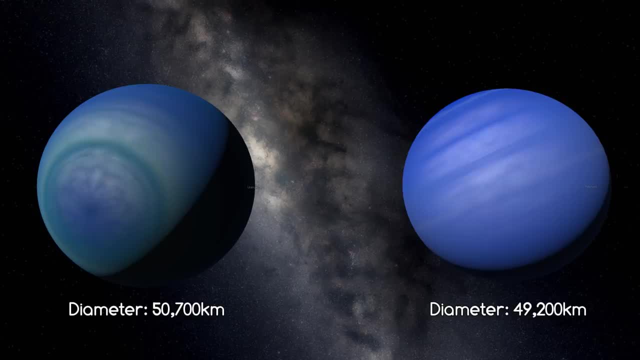 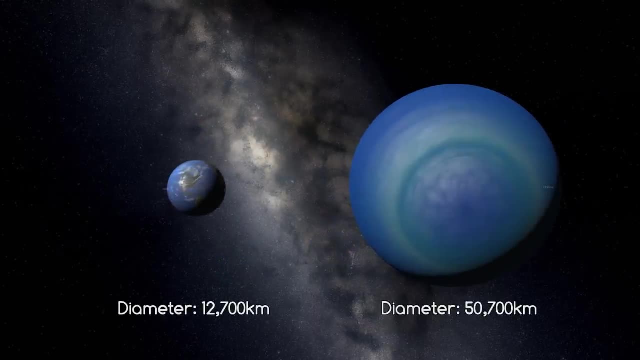 Earth masses. Its diameter, though, It's just bigger than Neptune's at 50,700km, about 4 times more than Earth's. Because this mass is spread out over a large area, the gravity on Uranus is only slightly less than on Earth, at 8.7m per second squared, or 0.89g. 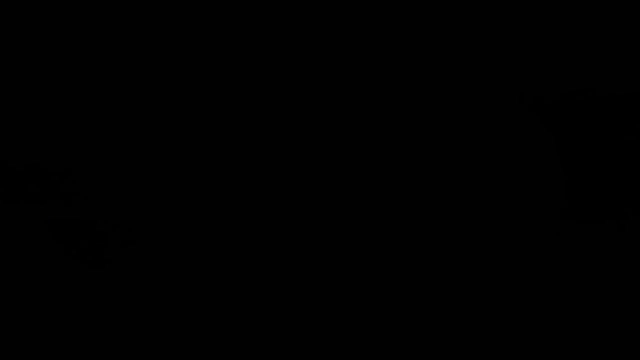 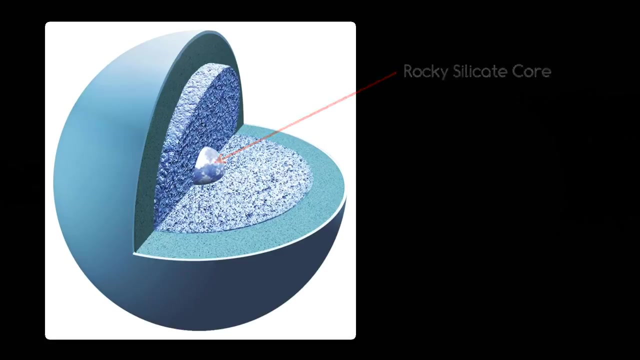 That would feel quite comfortable. And what is it made of? Well, it has a rocky silicate material smaller than Earth at the core. It is surrounded by a mantle of water, ammonia and methane- ices. Although it's referred to as ices, this mantle is in fact very hot, reaching almost 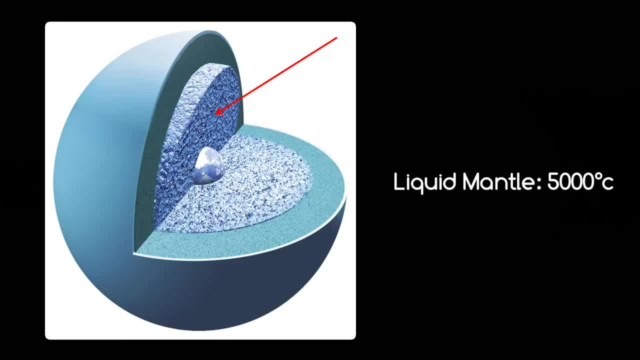 5,000 degrees centigrade and is more like a liquid ocean surrounding the core. The atmosphere is, in comparison, very insubstantial, only consisting of a total of 0.5 Earth masses, most of the mass of Uranus being in the core and in the mantle. 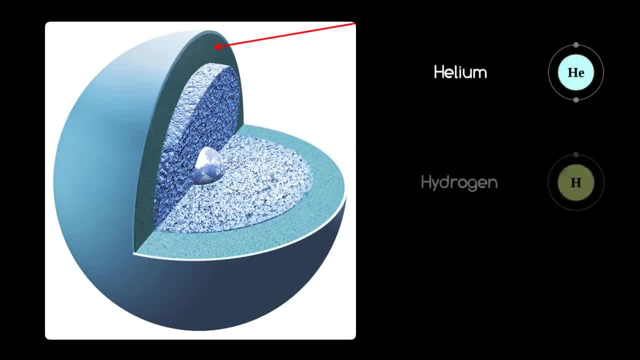 The atmosphere is quite large, but it's not a big deal. The atmosphere is quite large, but it's not a big deal. Uranus is comprised of mostly helium hydrogen and 2.3% methane, and then a cloud layer on. 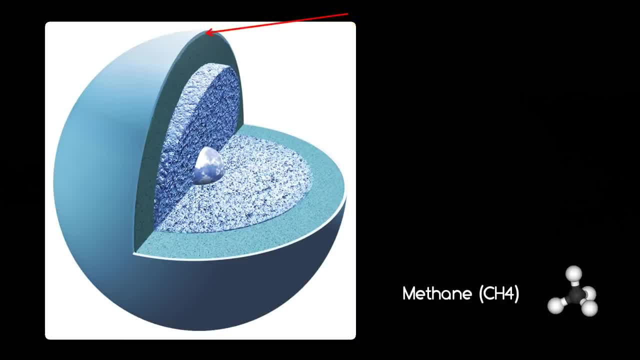 top. It's this methane that gives Uranus its aquamarine or cyan colour. Very interestingly, some models suggest that the pressure at the base of the mantle on Uranus is enough to break apart the methane molecules, which then compresses the carbon. 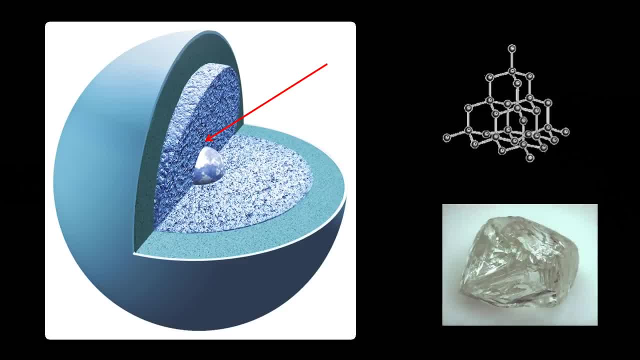 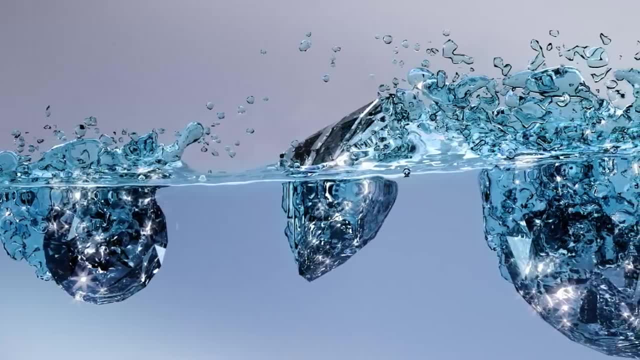 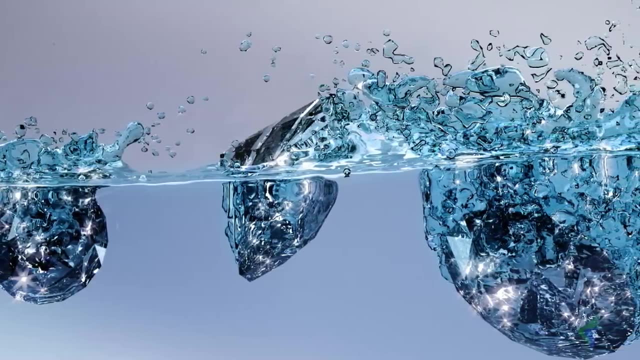 atoms from the methane into diamonds. These diamonds rain through the mantle Unbelievably. the very base of the mantle could be a layer of liquid diamond, with solid diamond bergs floating in it. To me that's a bit difficult to wrap my head around. 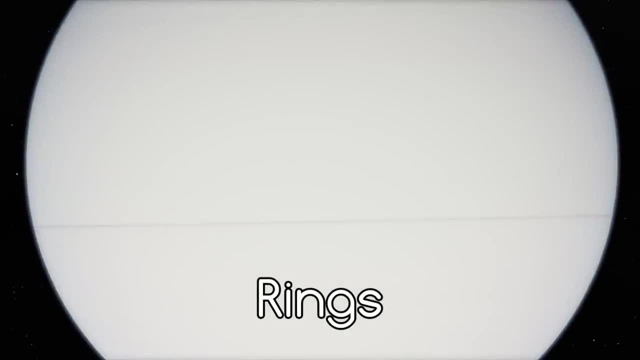 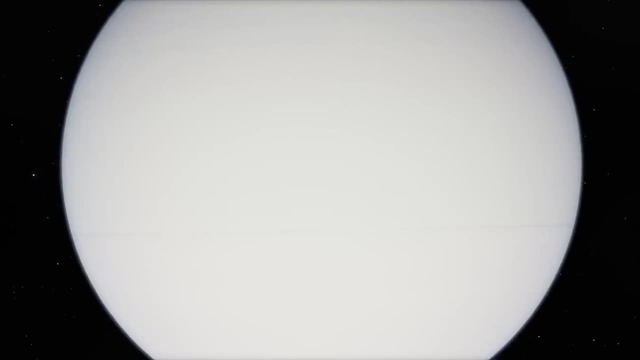 We'll fly away from the planet just a little bit now to have a look at its planetary ring system. Uranus, much like the other large planets in our solar system, has rings. It has 13 very dark and young rings. This means that Uranus has 13 very dark and young rings. 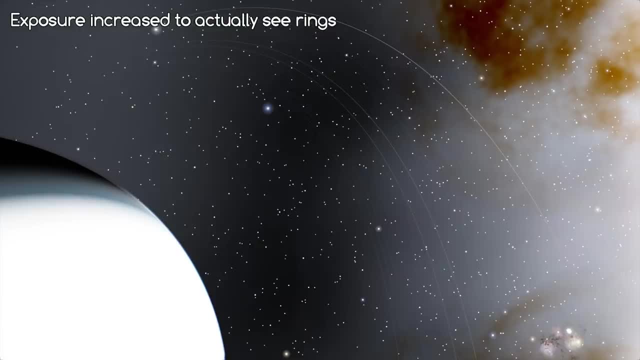 This means that Uranus has 13 very dark and young rings. This means that Uranus has 13 very dark and young rings. Most of them are not wider than a few kilometres and they are thought to only be 600 million years old, much younger than Uranus. 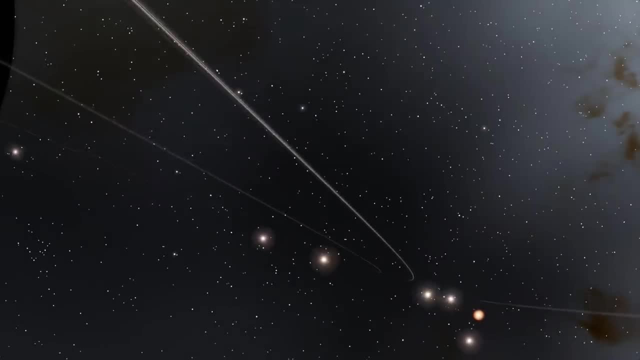 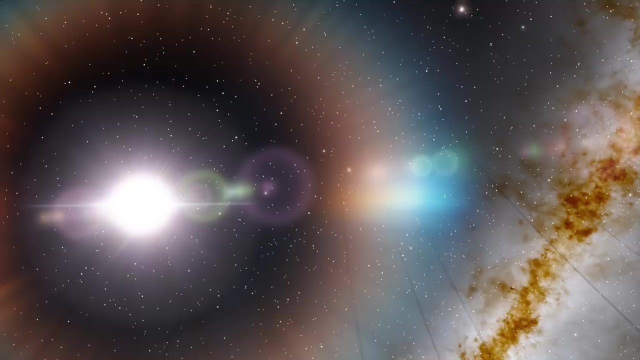 They are comprised of extremely small particles, the biggest being only a few metres across, made of water, ice and dark radiation-processed organics. Their albedo doesn't exceed 2%, or in other words, darker than wet soil, As we will see shortly. we will have to wait and see. 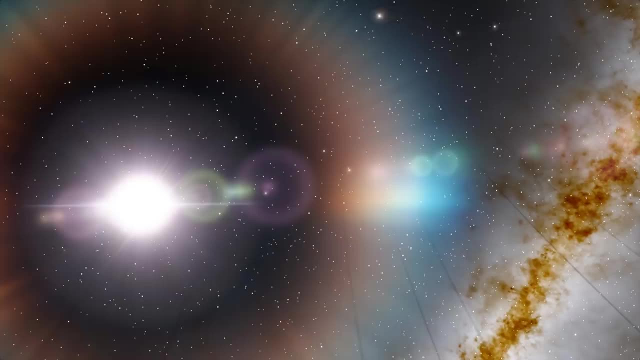 We will have to wait and see. We have to wait and see, We have to wait and see, We have to wait and see. Uranus has a lot of moons and the rings are thought to be the result of high-impact collisions. 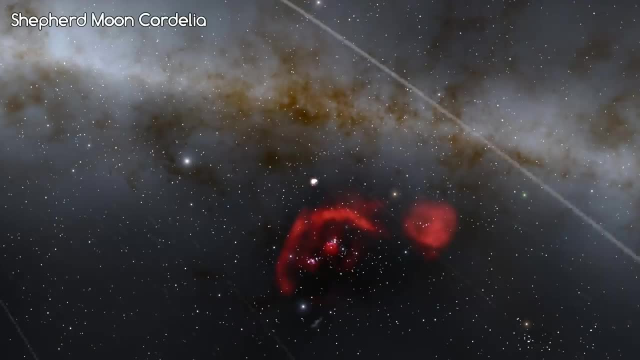 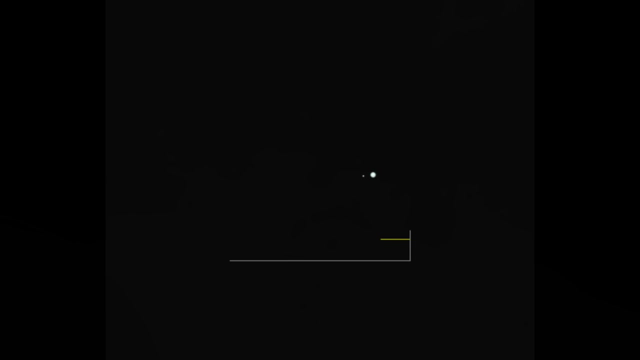 of some moons in the past. It is unclear why some of the rings are kept so narrow, the usual explanation being that rings are kept in line by shepherd moons, but this is only the case for one of the rings. Uranus was discovered to have rings in 1977, when an occultation of a star occurred. 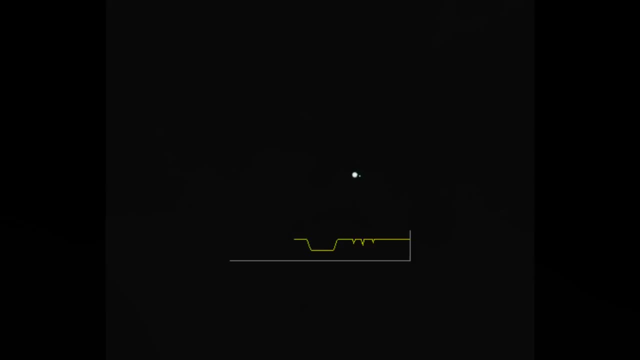 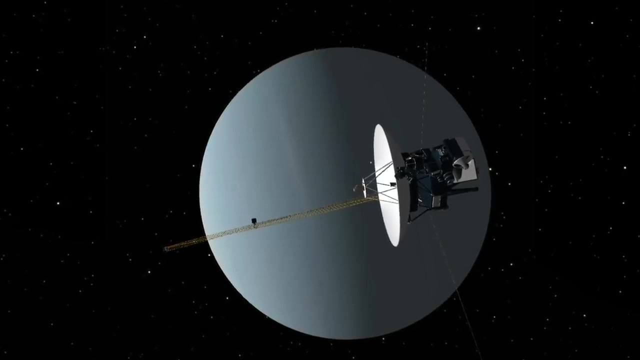 The star dimmed a few times on either side of Uranus, Uranus, as Uranus moved in front of it, confirming the presence of rings. Uranus has only been visited by spacecraft once, that was in 1986 by Voyager 2.. Voyager 2 discovered a lot of. 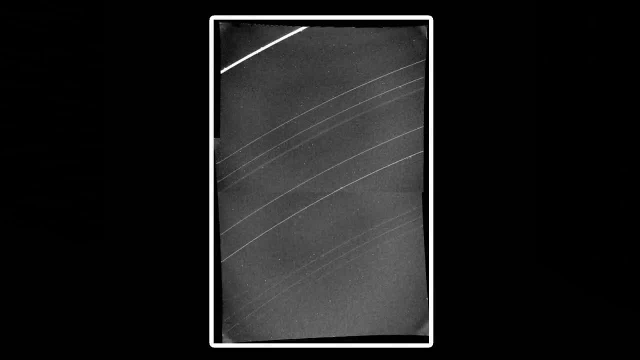 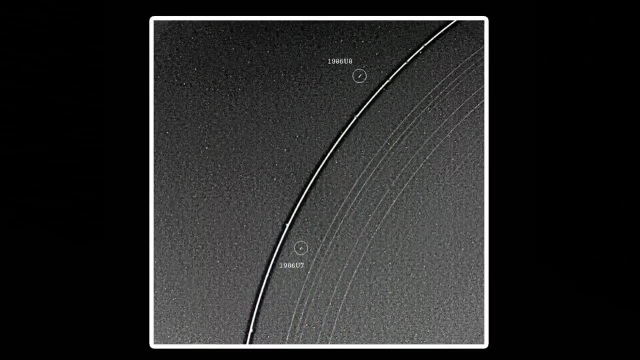 the rings and moons of Uranus, giving us close up shots of the faint ring systems. When Voyager flew by, though, this only brought the total of known rings to 11.. When Helper was launched, it also had a look at Uranus. discovering two additional rings that had never been seen before. The outermost ring is twice as far away from Uranus as the previously thought outermost ring And, as promised, here is a look at the many moons. Unusually, the moons are named after figures in English literature. 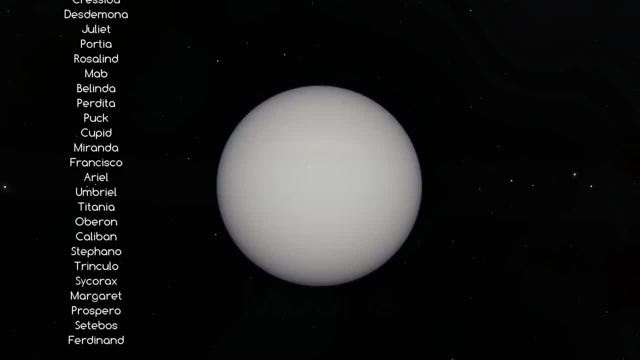 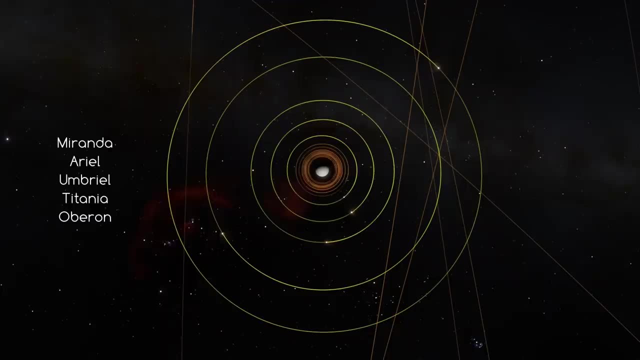 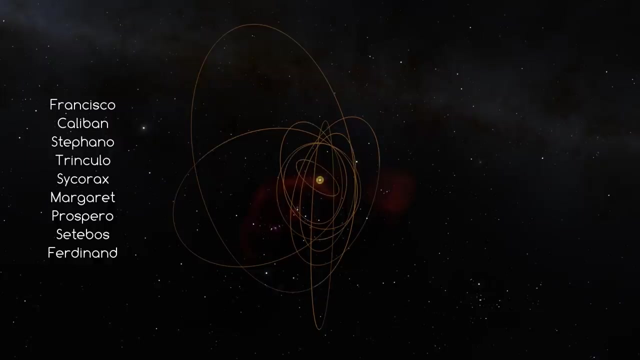 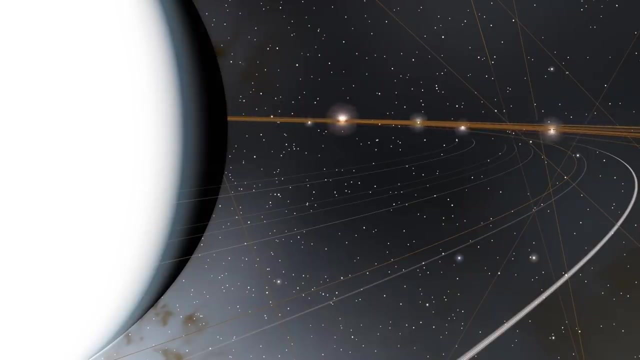 Overall, Uranus has 27 known moons, divided into 3 categories: The 13 inner moons, the 5 major moons and the 9 irregular moons. The inner moons are connected with the rings of Uranus, some of which may have provided the ring. 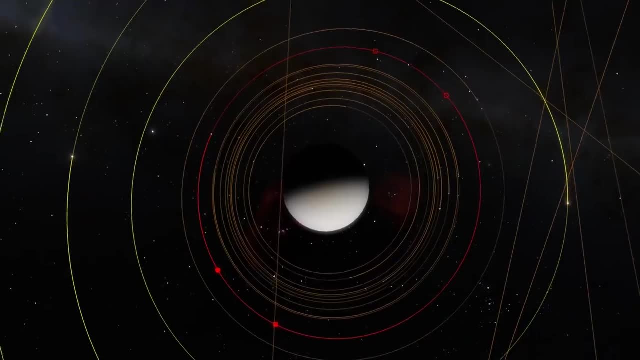 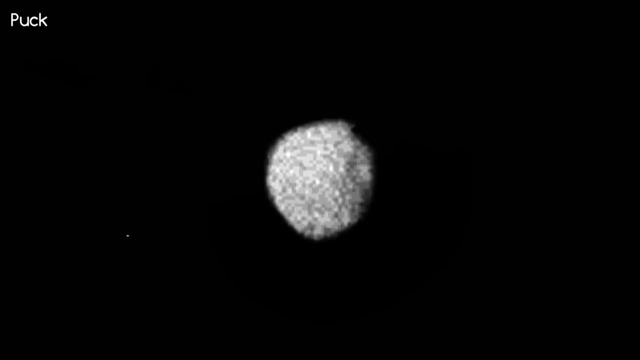 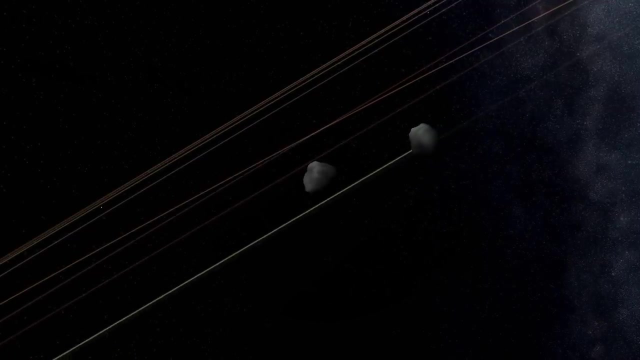 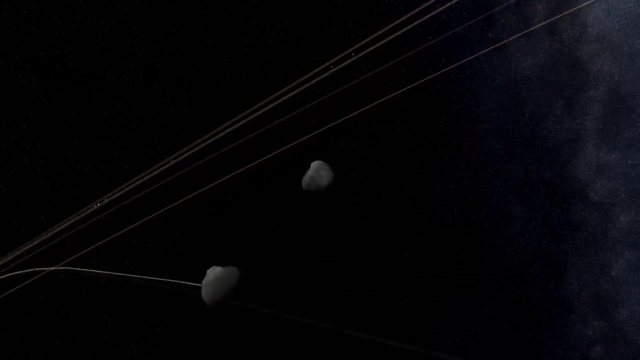 materials. The largest of these moons is called Puck, at only 162km in diameter. It is the only of the inner moons to be captured in detail by Voyager 2.. Interestingly, these inner moons constantly perturb each other and the system seems very unstable. There's a good chance some of them may collide again in the future. 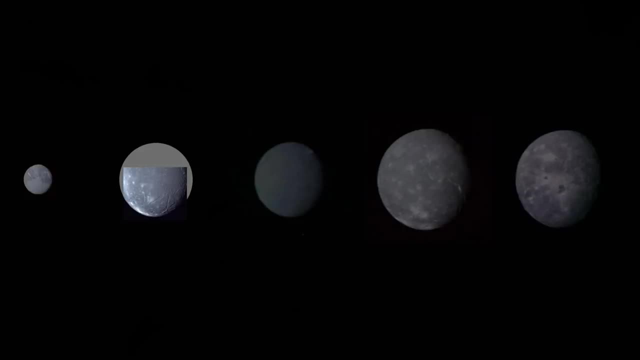 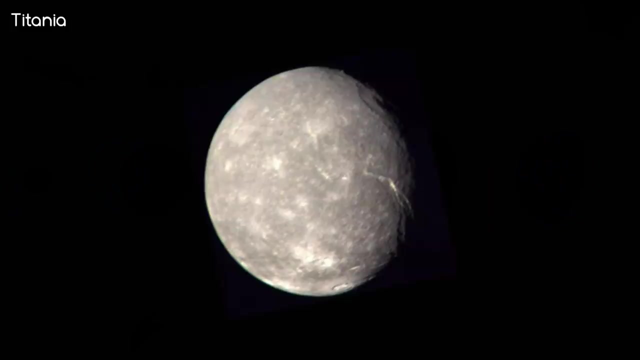 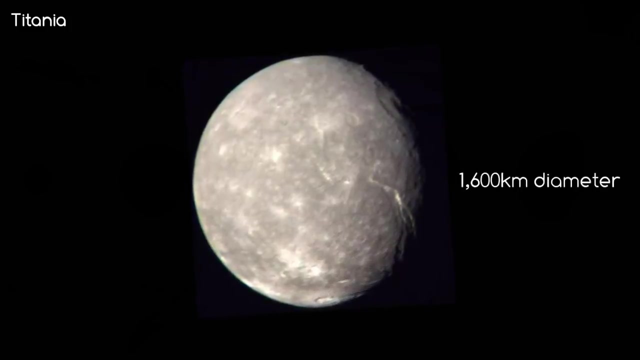 The 5 biggest moons, in order of distance from Uranus, starting on the left, are Miranda, Ariel, Umbriel, Titania and Oberon. Titania is the largest moon of Uranus and the 8th largest moon in the solar system, at 1600km in diameter. 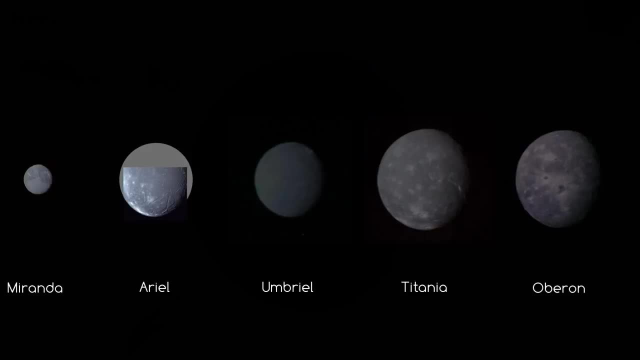 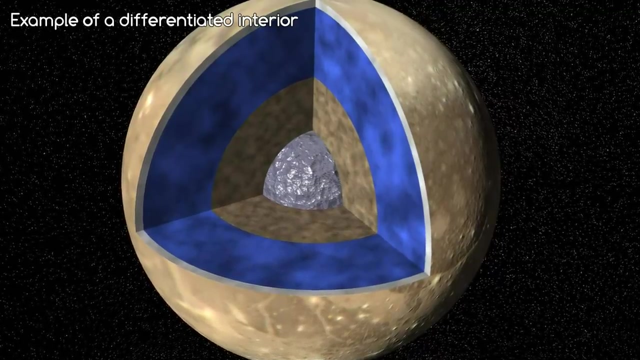 Again, as can be seen, these are very dark objects, Umbriel being the darkest, With the exception of Miranda, which is comprised mainly of water ice. the rest are thought to be a mix of water and rocky materials. These moons may have differentiated interiors, meaning a core of 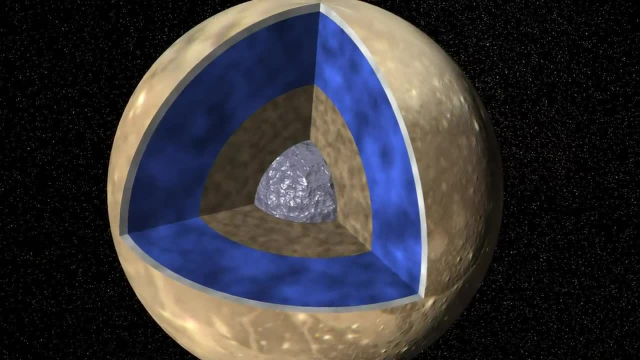 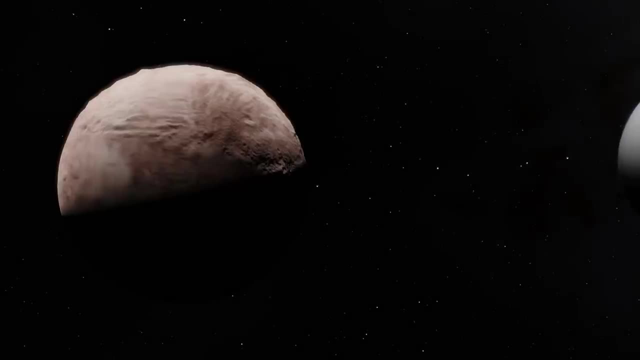 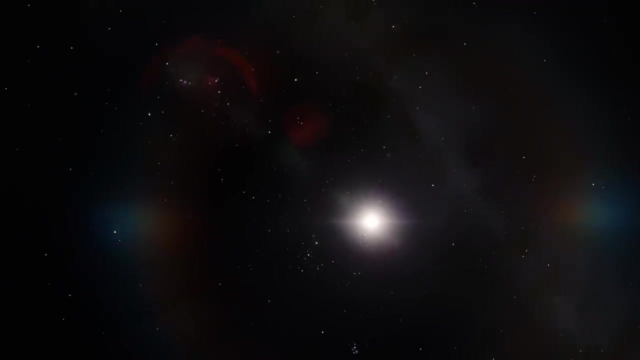 rocky material with a mantle of ice Between the core and the mantle could well be an ocean of liquid water. Interestingly, the axial tilt of the large moons is the same as Uranus, meaning that during solstice, if you were to look at the sun, 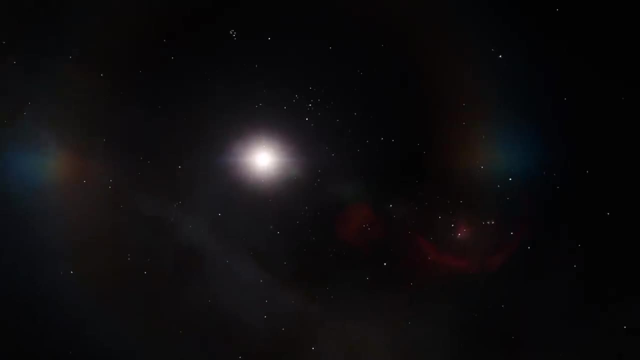 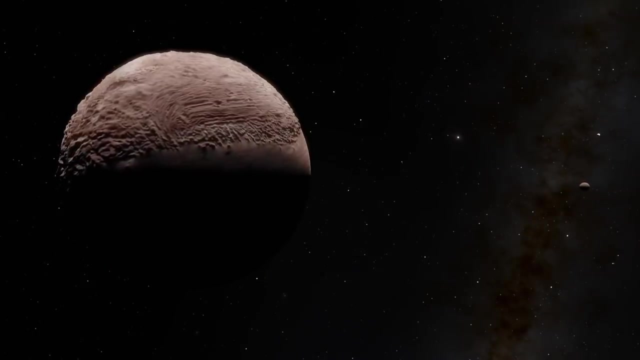 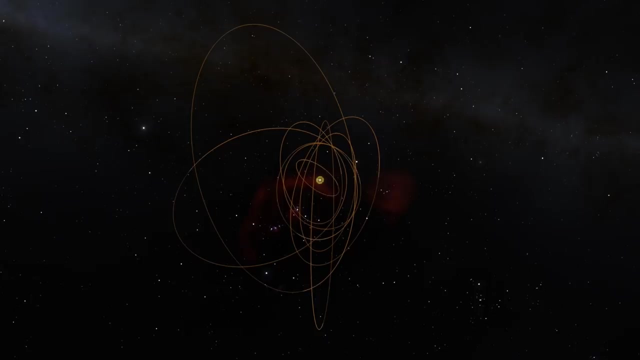 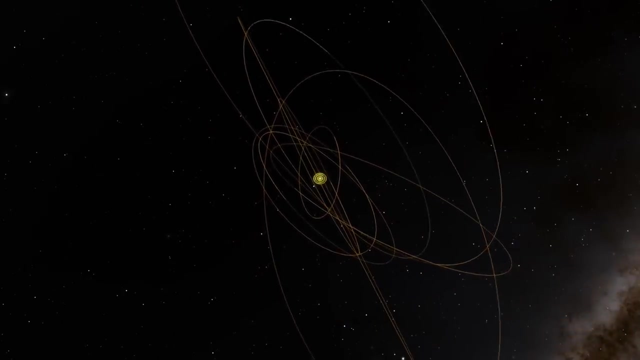 it would only ever move in a circle in the sky never setting. During solstice, only one side of the moon faces the sun, meaning constant daytime. The final 9 moons are irregular moons. They are likely to be captured objects and are much further out than the last of the big moons. 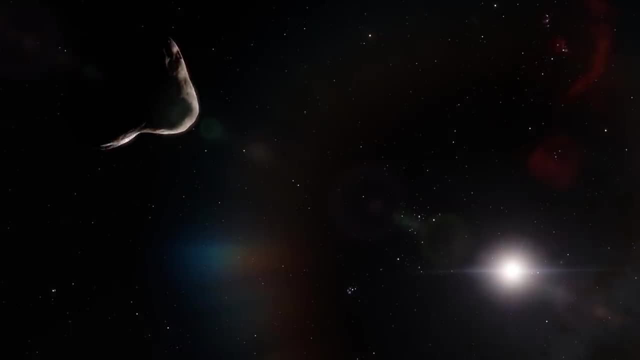 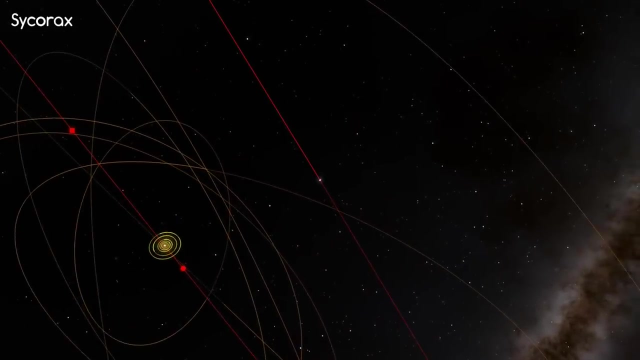 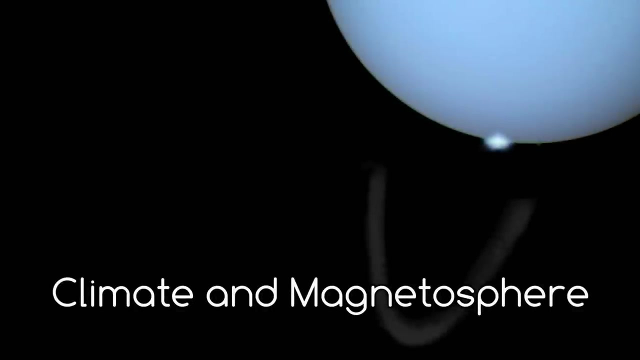 Oberon. They vary in size, from 20km to the biggest Sycorax, which is 200km in diameter. Exploring Uranus. Exploring Uranus. Finally, let's explore Uranus' climate and magnetosphere. Uranus' seasons are quite unique in the solar system due to its 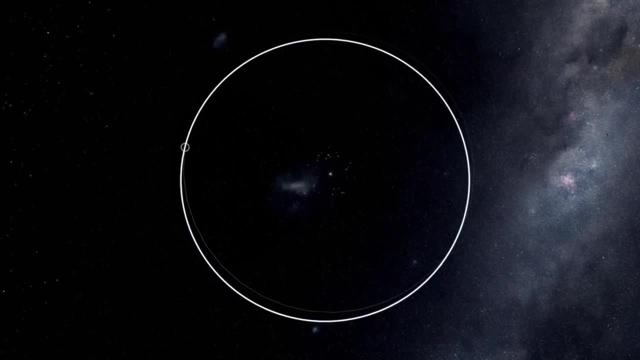 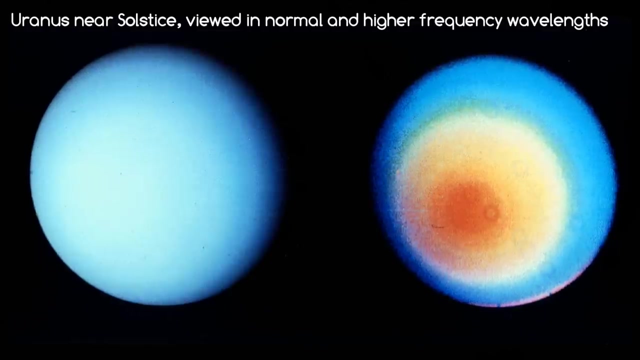 exceptional axial tilt. We only have data for about one Uranian year, though, which means it's difficult to be able to say with certainty differences between the years. What has been observed is that, as the planet approaches solstice, the pole brightens and a collar forms Moving away. 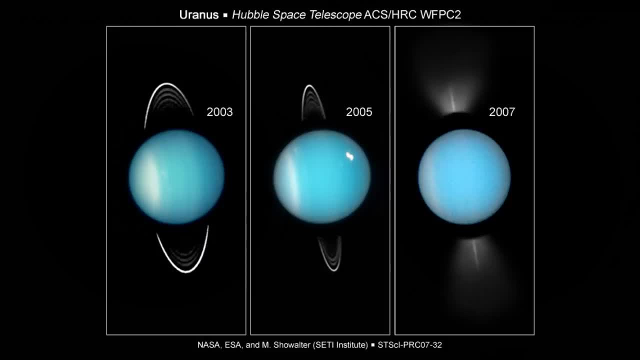 from solstice, the pole and the collar form. Moving away from solstice, the pole and the collar form the pole and the collars dim. This brightness is thought to be because of the thickening of methane clouds, although the cause is not clear. Seasons also affect storms in the upper 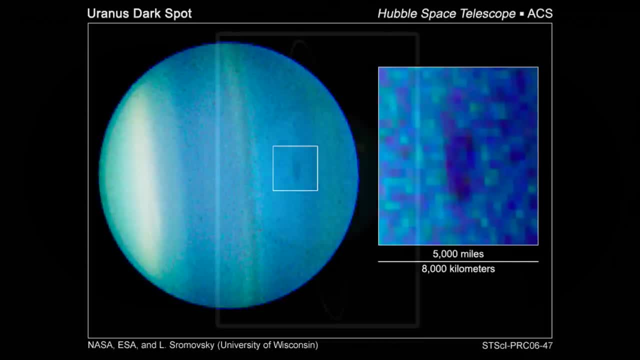 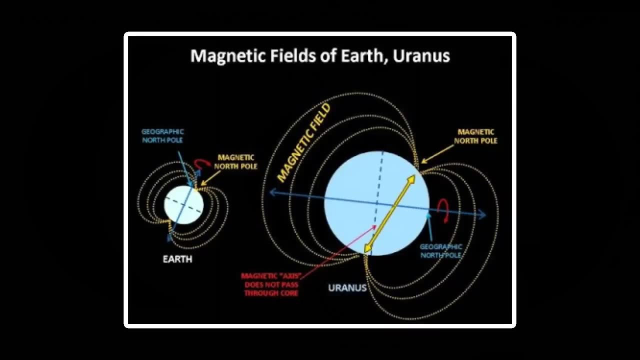 atmosphere. Storms are relatively rare on Uranus compared to the other gas giants, but are thought to be caused by changes in the seasons. And another unique feature of Uranus is its unusual magnetosphere. Usually, magnetospheres originate from the geometric centre of the planet, but that's not the case with Uranus. Also, it's not in line with the rotational axis, but 59 degrees off. This unusual placement means the magnetosphere is much stronger at the north pole than at the south. One theory for this is the liquid diamond ocean could deflect the magnetosphere, or even that it. 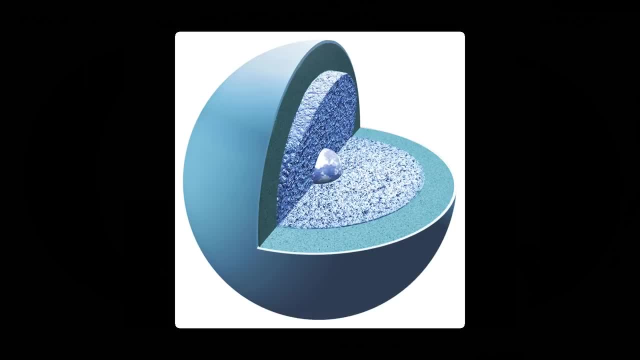 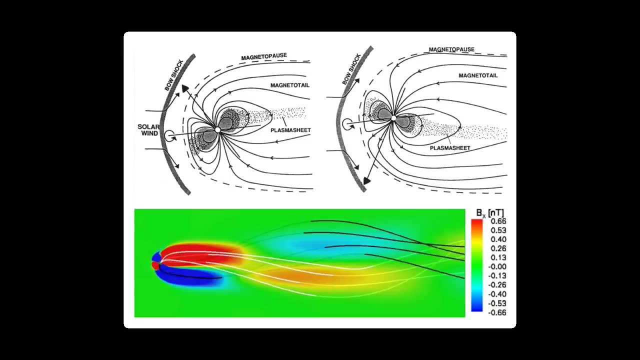 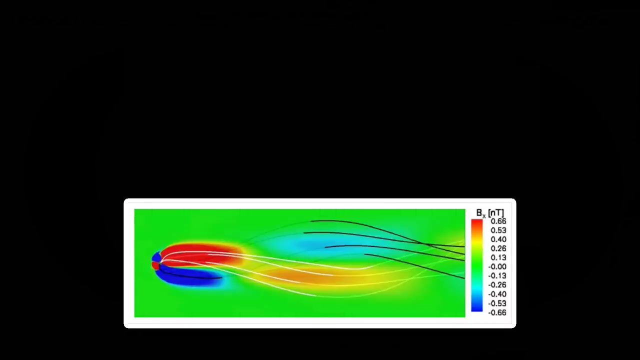 is not the core of the planet that produces the magnetosphere in the future. The magnetosphere is about as strong as Earth's and because of its unusual rotation, the magneto-tail corkscrews off for millions of kilometres into space. 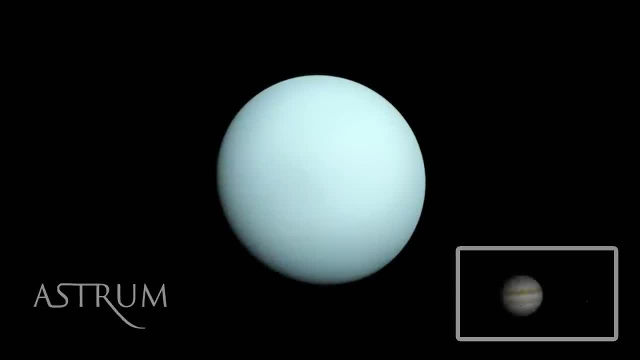 Well, thank you so much for watching. I hope you've learned more about this rather mysterious planet. I was dreading making this video a bit, because I was wondering if there were any other planets in the world that could be as strong as this planet. I hope you've. learned more about this rather mysterious planet. I was dreading making this video a bit because I was wondering if there were any other planets in the world that could be as strong as this planet. I was dreading making this video a bit because I was wondering. 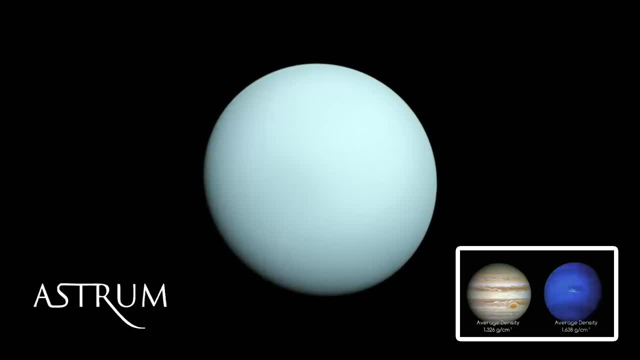 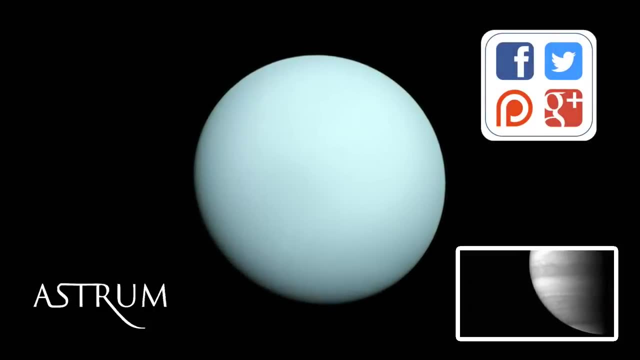 what I could actually talk about. Having done the research, though, I found it one of the most interesting planets I've actually covered so far. If you want to support what I'm doing here, then I have social media links that you can follow, and I've also started. 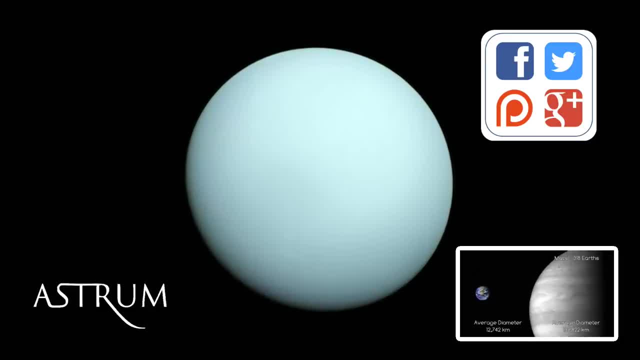 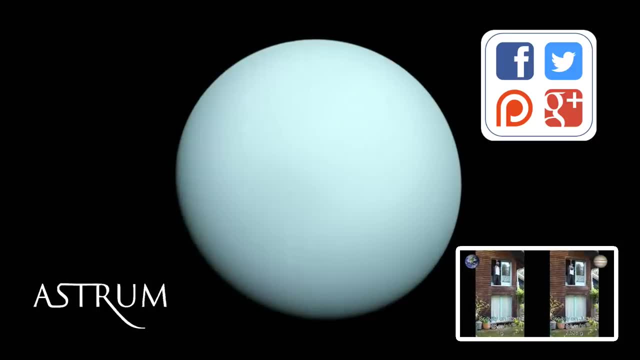 a Patreon page if you wanted to donate to the videos I'm making. Finally, I've made a lot of other videos on space and other planets you may be interested in, so be sure to check them out. See you next time.